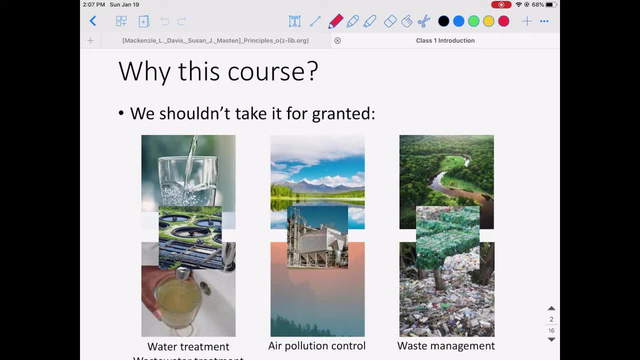 clear sky. this is fresh air, okay, and i think the air quality in Rolla is also pretty good, so we don't have a lot of those polluted days there and we can also enjoy these very good weather, very good air, and also we have these very clean soils where a great forest can start to grow on. 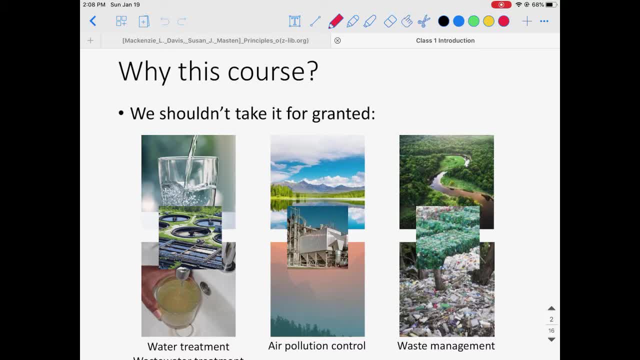 them, a lot of plants can live, i would say, happily on these soil here. but we should- shouldn't take these for granted because they don't happen. these things actually happen at a price. if we don't properly manage our environment, they can easily turn into these results. okay, so the clean water. 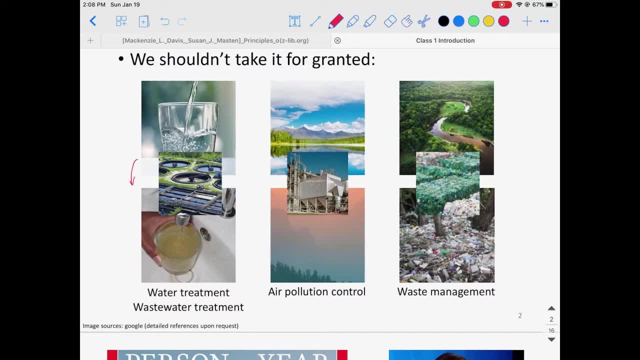 can get contaminated. okay, you can see that sometimes, or in very rare cases, when we turn around the tab, water coming out is brownish, and this is not very old stories actually. in 2014, there's a flint water crisis where people discover a lot of toxic materials in the drinking water. 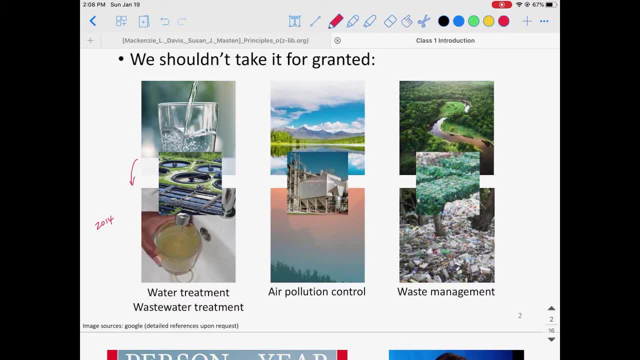 okay, and also in terms of the air. in more divided countries, let's say in the us, in canada or in the european countries, the weather or the air indeed looked like this, but in a lot of developing countries or in a lot of the major cities, we're seeing observing serious 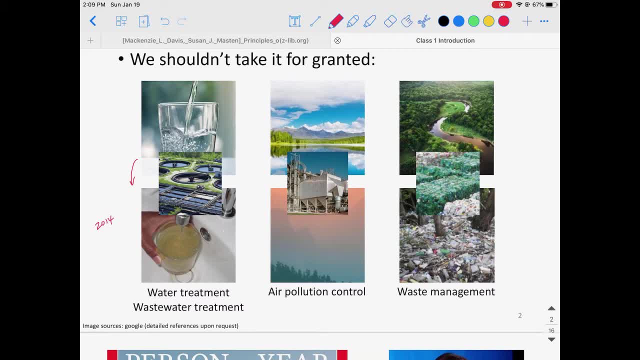 air pollution problems there, where the sky looks very hazy and people with allergies or people with some other diseases are going to be very sensitive to these environments. and further, in terms of the soil, we can easily turn these clean soil into these contaminated soils, but just dumping trash is everywhere and we have to also notice that the trash contains a lot of. 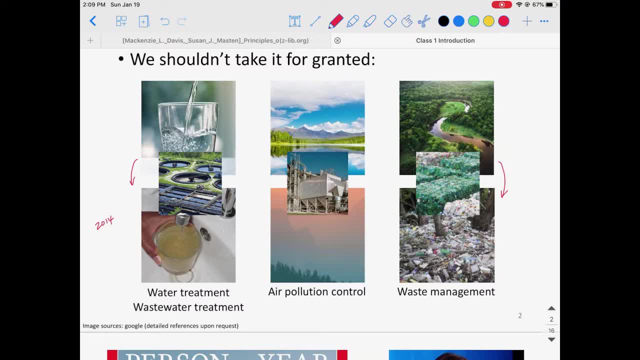 pollutant- pollutant species like toxic materials and they can get leaked into the soil system. that's going to finally harm the plants in the soil system. so we have to do a lot of or manage a lot of these environmental issues with methods, okay, with some techniques. we call these techniques. 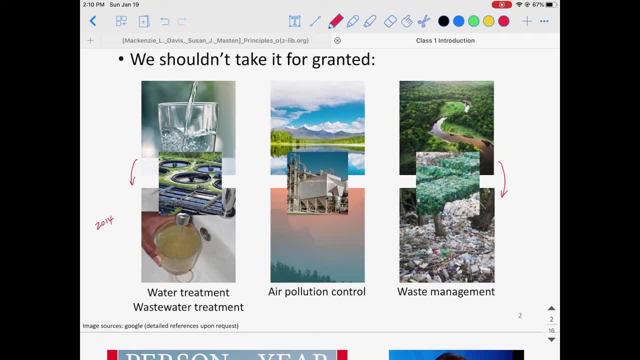 belong to the environmental engineering, for example, in water system. you know we have the water treatment for producing the drinkable drinkable water, potable water- okay. we have the wastewater treatment to deal with the waste water that's coming from the industry or coming from the residential areas. okay, to treat them before we release them back into the environment. 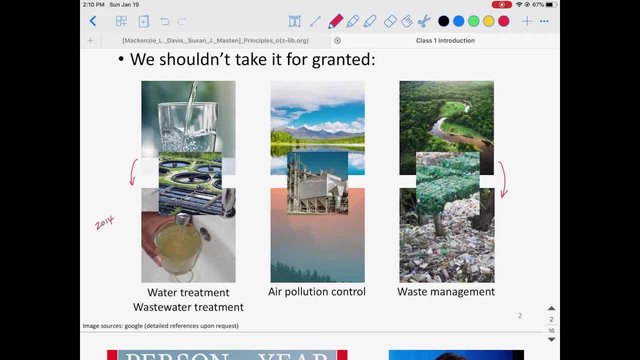 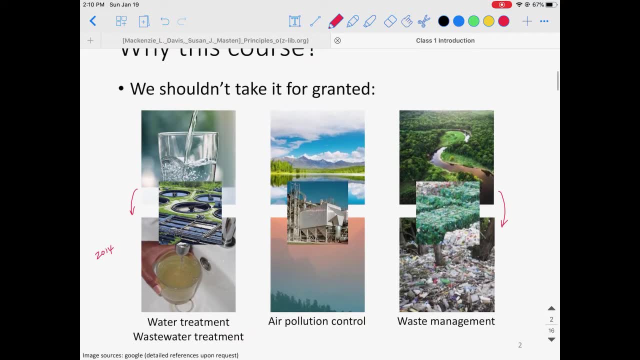 and for the air. we need to do air pollution control. you can design a lot of pollution control. you can design a lot of devices to get rid of these pollutant species in the air. in terms of soil, we need to do soil or the solid waste management right to pack these. 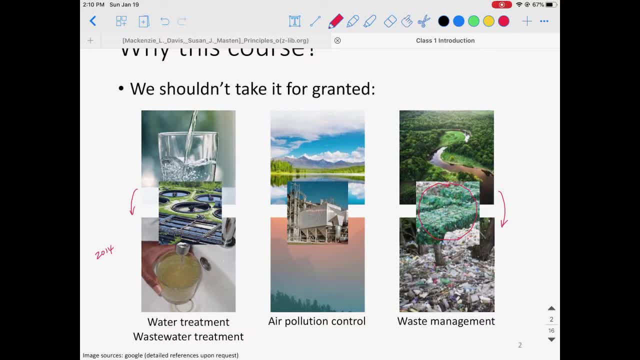 trash with specific categories and then further process them with the corresponding materials, and you can see that there are a lot of these environmental issues in almost all different areas. so let's think about what are the states of the matter. states of the matter: okay, they can exist. 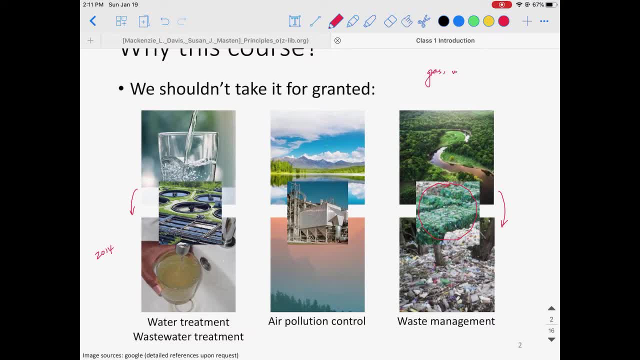 in the gas phase, okay. the liquid phase or in the solid phase, okay. so you can see that these environmental problems can happen in all of these, uh, different phase of the matter. so the environmental engineering tries to solve all of these, or at least try to mitigate these environmental problems, okay. then you may wonder: why don't we just 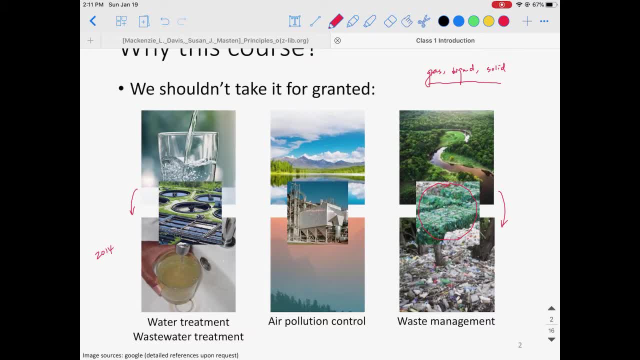 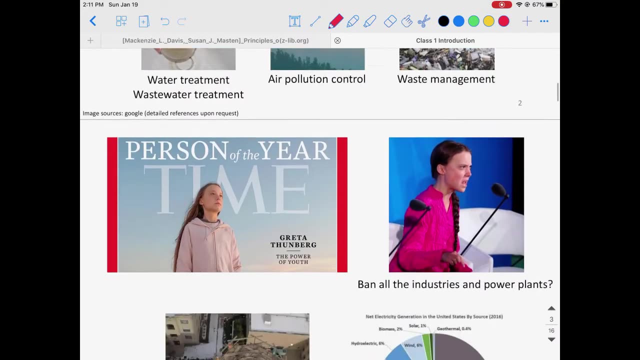 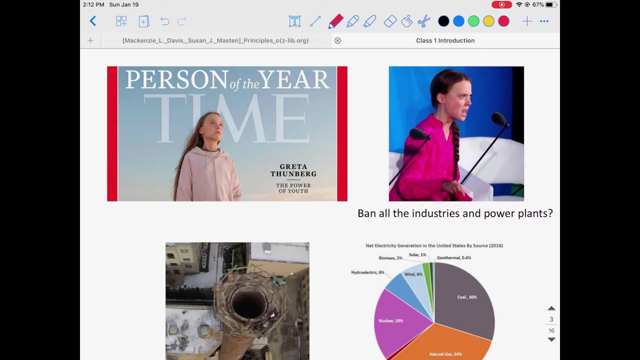 don't produce all of these, all of these pollutants, in the beginning? why don't we just leave without requesting all the sources, all the resources from the environment, or not producing any pollutions at all? there are indeed some people trying to advocate these lifestyles, so this is especially the case for the younger generations, and i'm sure that some of you. 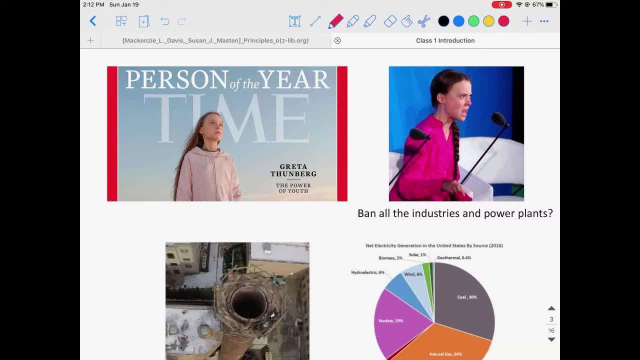 in the class are also wondering about this. why can't we just learn in a natural way, like the caveman? okay, so i'm pretty sure that you are quite familiar with this girl here, greta thomberg, so she's a quite active person that's advocating or raising the 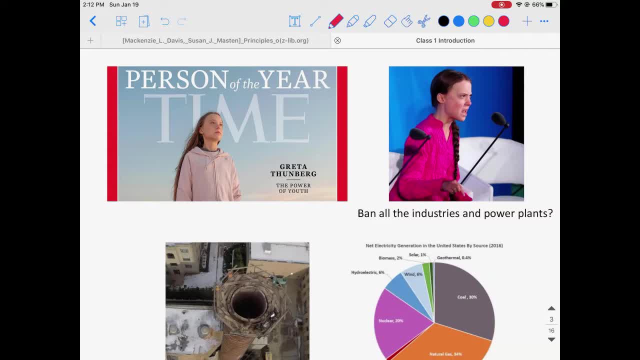 awareness of the these environmental problems that's happening on earth right. so she may also made a speech in the united nations right calling all of the countries to realize these environmental issues and to protect our planet. so during these advocates or during these activities, people are promoting or people are proposing that we should ban all the industries or 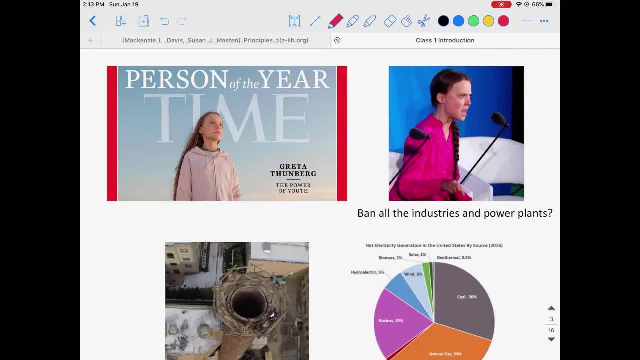 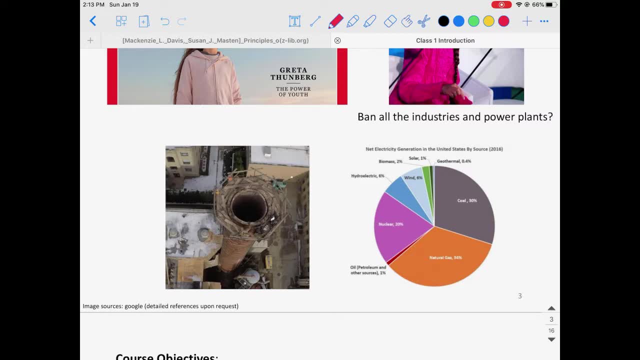 ban all the power plants and actually i'm quite happy to see that our school, msrsmt, is actually making a positive move here. so, as you have noticed, our school have already discommissioned the coal-fired power plant and actually we dismantled this chimney from the power plant. 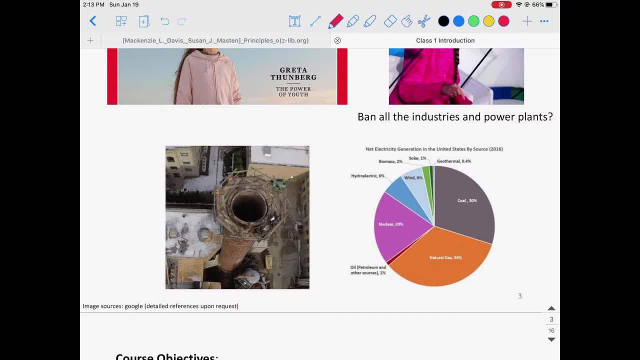 during the winter break, okay, and instead of using the electricity coming from the coal-fired power plant, we converted. we basically started to take the energy from the geothermal that's available in our school. okay, so this is a very active step actually to convert our reliance onto the fossil fuel combustion. 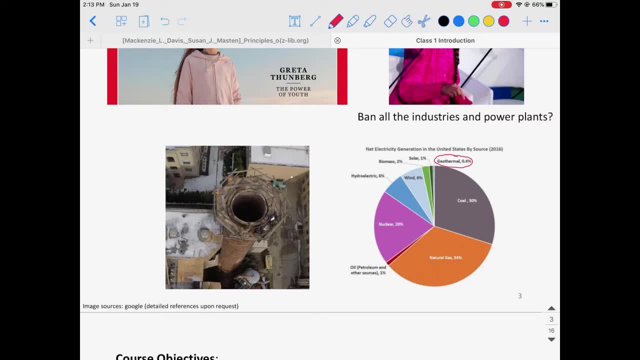 into these renewable sources, but if you take a look at the electricity generation in the united. So this is data coming from 2016,, which is three years ago, and I have to say that the pie chart will somewhat look quite similar, although the detailed numbers might change. 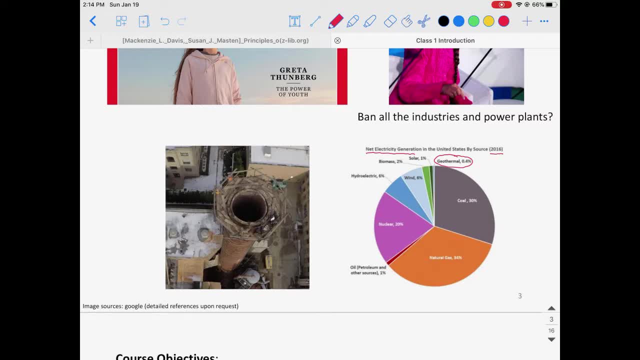 a little bit. So what you can find out is that actually, coal is still taking around 30% of all of this electricity production, Although there are other resources of natural and renewable energies, for example hydroelectric, biomass, solar, wind, geothermal, et al. 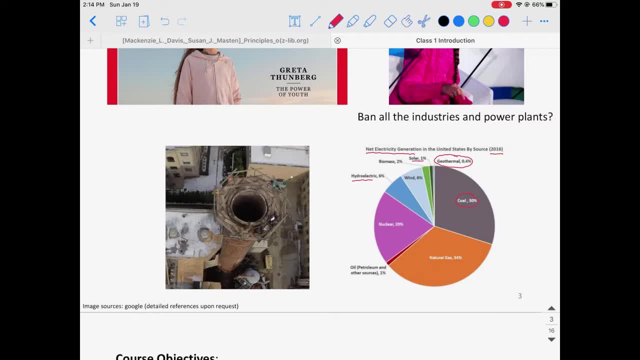 But we're still strongly relying on the fossil fuel, especially coal combustion. There's no easy way for us to cut all of these coal supplies, cut all of these coal-fired power plants And then transition, And then transition into these renewable energies. 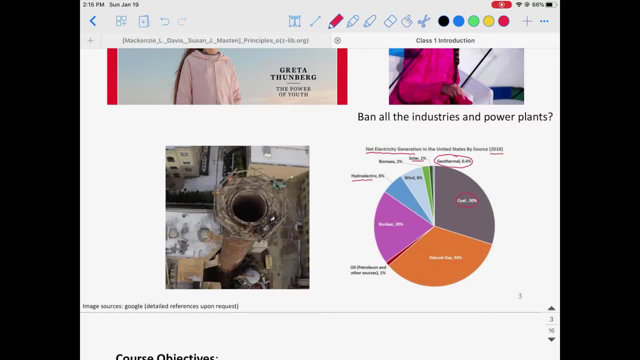 And, in addition, these renewable energies are not as reliable or as stable compared to these coal-fired power plants, For example the solar energy. So typically during the night the electricity demand will see a spike because people return to home. You don't have a lot of lighting right. 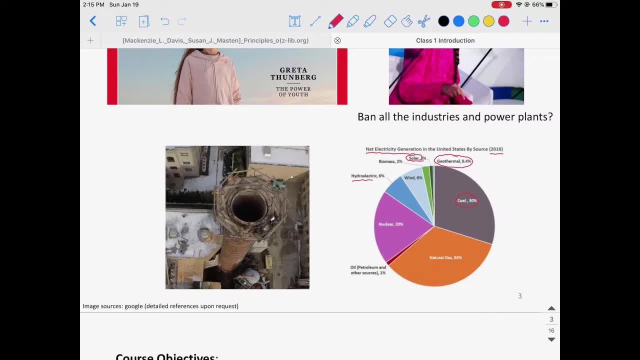 You don't have the solar radiation to provide you with the light there. So basically the energy demand, It will spike up overnight. What this means is that we'll need more electricity production at that time. We also note, and we also know that the solar energy overnight basically is zero right. 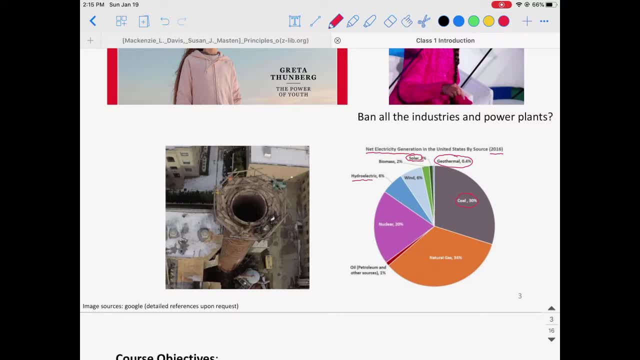 There is no way we can produce the solar energy here. Another example is wind, because there's a very unstable wind resources at any location. Who knows? There is no way that the wind is always blowing at the same speed over 24 hours over the. 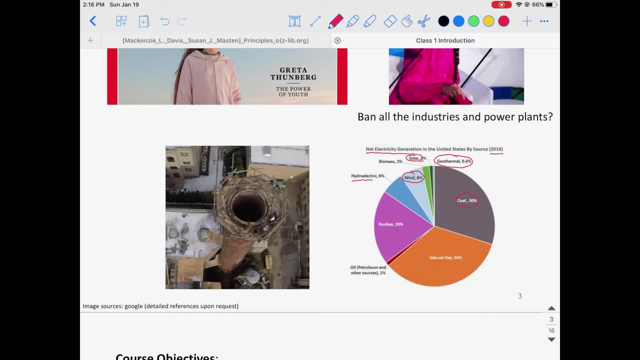 entire year, right? So we have to consider all of these instabilities in the electricity production. There is still a long way to go for these renewable energies, So that's why they're not even comparable to the coal-fired power plant. because we can. 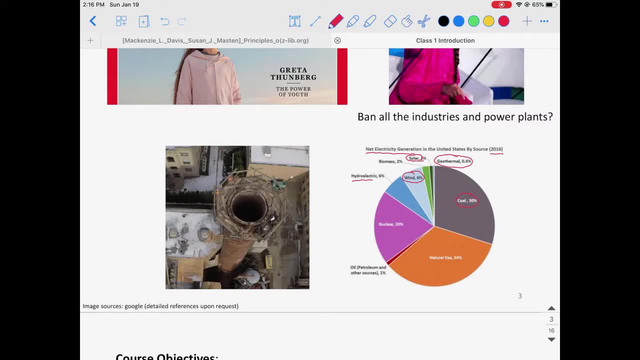 almost have endless production of the coal. So that's why they're not even comparable to the coal-fired power plant, because we can almost have endless production of the coal Right, And then we can always run the coal-fired power plant 24 hours over the several years. 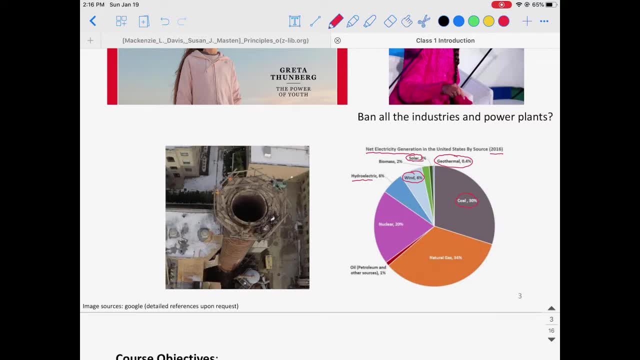 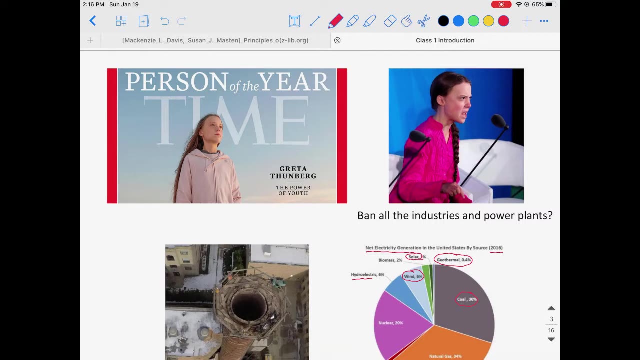 and we can easily generate a large amount of energy just by a few power plants in the United States. So there's no easy way for us to solve all of these environmental problems by just thinking about cutting all of these, Right? Okay, So we're cutting all of these energy productions here. 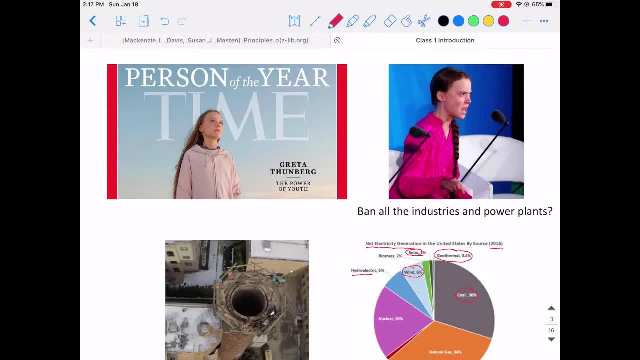 Okay, So through this class you will start to realize what are the basic principles in designing these environmental engineering devices to solve the problems in water treatment, wastewater treatment and also air pollution. Okay, So you will realize what is the scale we're talking about and what are the designing principles. 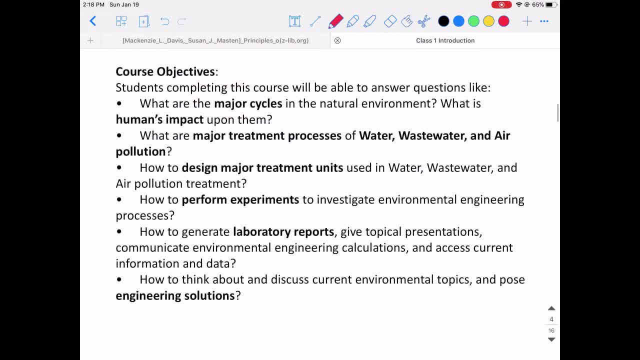 for these devices. So here is an overview of the course objectives. So you guys, after the completion of this class, you should be able to answer questions, for example like: what are the major cycles in the natural environment? what is the human? 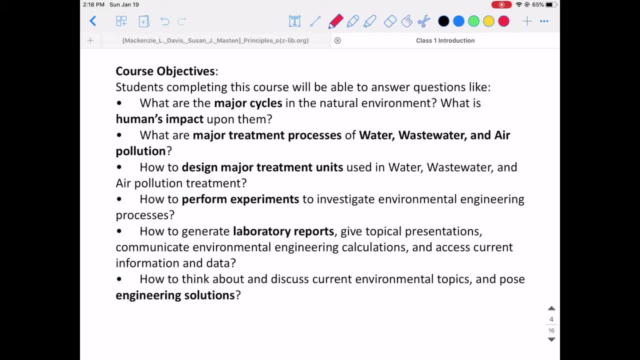 impact upon them. And also, what are the major treatment processes for water, wastewater, air pollution? Okay, how to design major treatment units used in water, wastewater and air pollution treatment. so you can see that we're basically water and air pollution are the major problems we're trying to deal with right now, and also how to perform. 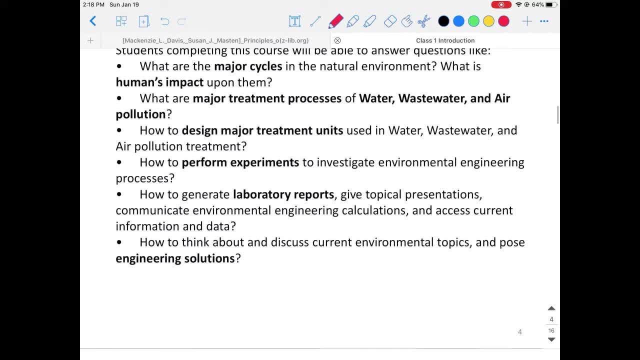 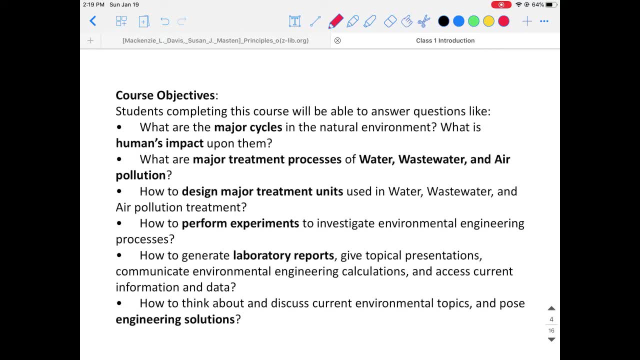 experiments to investigate environmental engineering processes. so, as you have might have noticed, for this class we are also having a concurrent experimental section, so you are going to learn about the basic ideas- how to do environmental sampling, how to design or these environmental devices to deal with the pollution problems, and you should be able to know how to generate laboratory. 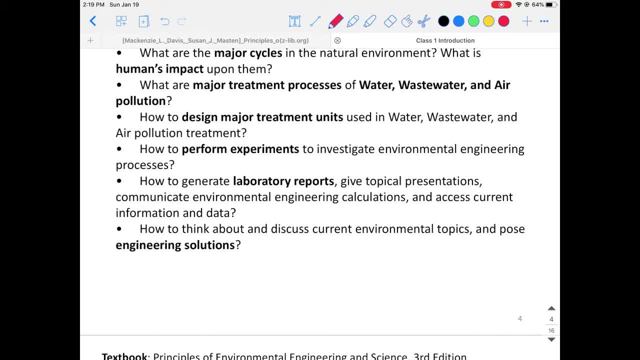 reports, give topical presentations, communicate with others and also work on solving these problems with mathematical calculations. okay, finally, I want to want you guys to think about and to discuss current environmental topics and post corresponding engineering solutions, not just by just saying that why don't we just cut all of the coal-fired power? 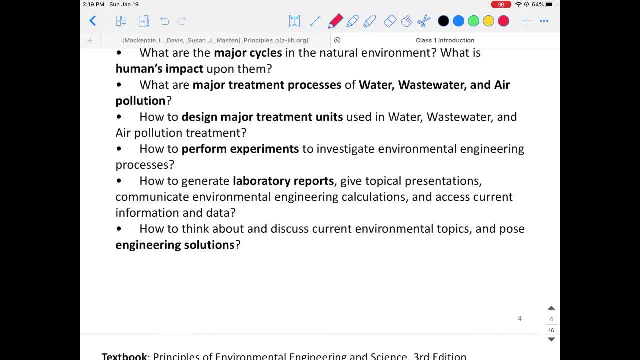 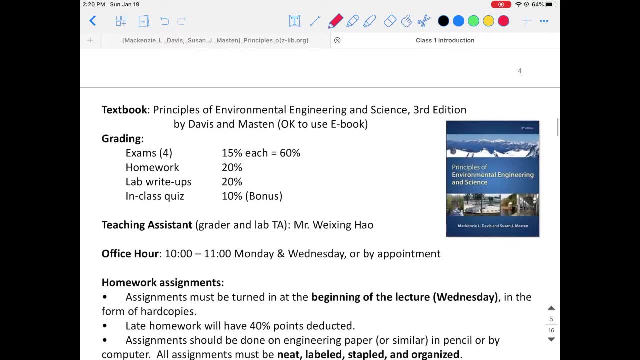 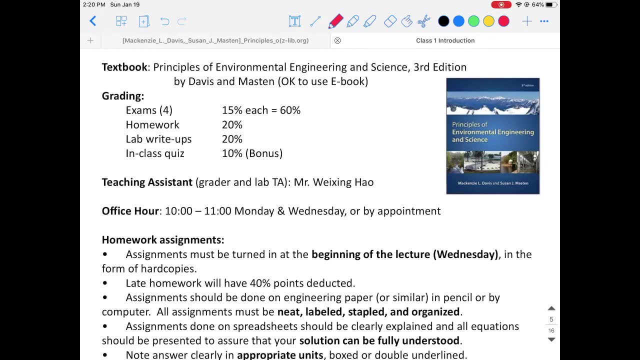 plants. okay so there's no easy way for us to directly transition into another treatment process there. okay so, in terms of the textbook? okay so, in terms of the textbook, we're going to use the principles of environmental engineering and science, the third edition by Davis and Mastin. so I noticed that this textbook already. 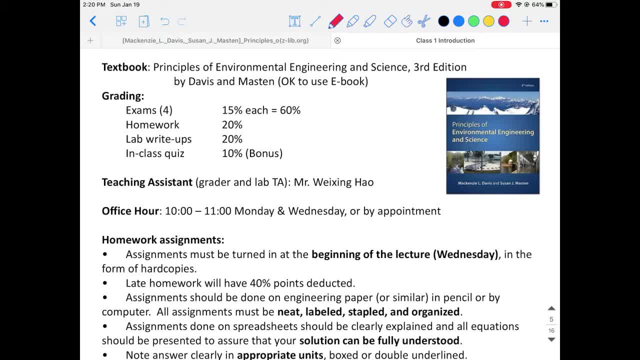 have the fourth edition, but right now is not in a very good binding condition, so when you order them, you're still going to receive them in loose pages. so, and since the third edition is still available on different websites and you can order the hard copies and also it's okay for you guys to use these, 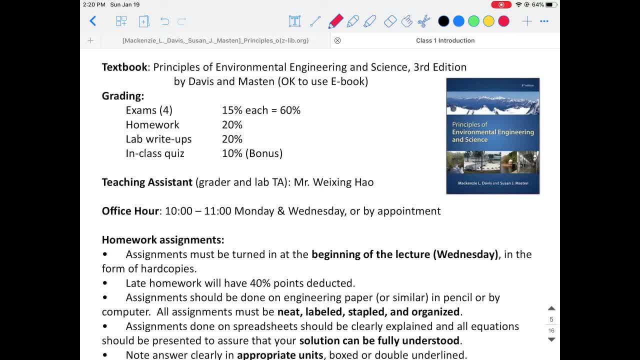 because for the exams they're closed book. but you can bring one page of the notes or basically the summaries. we can talk about that later, okay, so you don't have to. you cannot bring your textbook into the exam and for the textbook we are going to work on the reading assignments and also working on the. 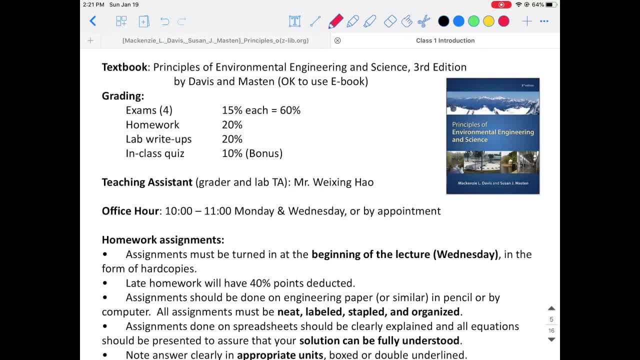 homework assignments. okay, and in terms of the grading, we're going to have four exams, so basically four quarters of the contents for this class. okay. so, because this is an entry-level environmental engineering class, so we're going to deal with quite many, quite many concepts and different treatment systems. okay, so I 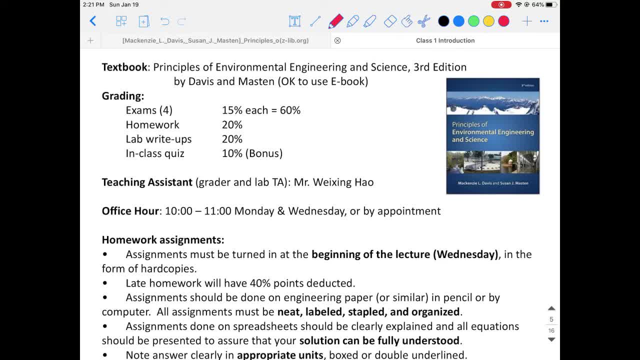 don't want you to want you to mix all of these concepts there, so it's probably a better way to take the exams every quarter so we can focus on certain topics and you can work on problems in these systems here. so for each of this exam is going to cover 15% of the scores. 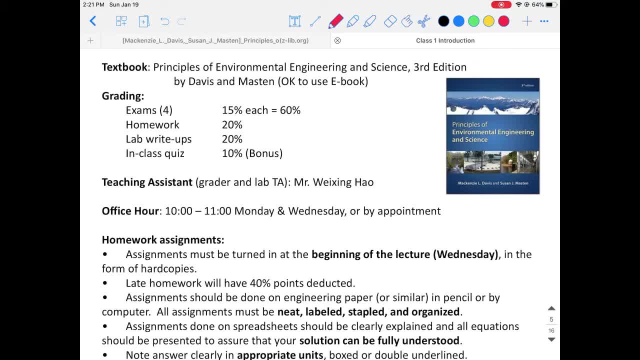 so four exams equals to 60%. okay. the homework covers 20%. the lab write-ups contains 20%. okay, and since these three items add up to 100%, so for the lab participant, for the class participation, I'm going to evaluate you guys with the in-class quiz and that's going to give you 10% bonus. okay, so you. 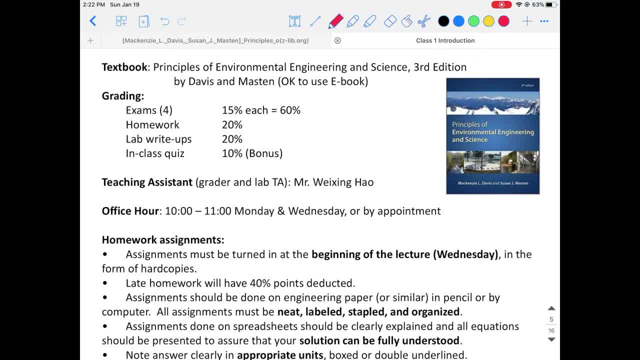 have to be in the class to fill in these quiz problems and you can get the bonus points. and the teaching assistant for this class is going to be Mr Wei Xinghao. okay, so he's also a PhD student in my lab. he's going to be the grader and also the 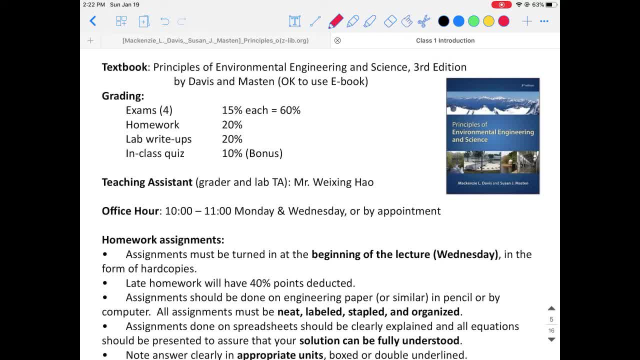 MPA for the class. okay, so if you have any questions, you can contact me or Wei Xing and we're happy to help you. so the office hour for this class is going to be one hour before the class. okay, so it's 10 to 11 every Monday and Wednesday, or you can set up appointment. 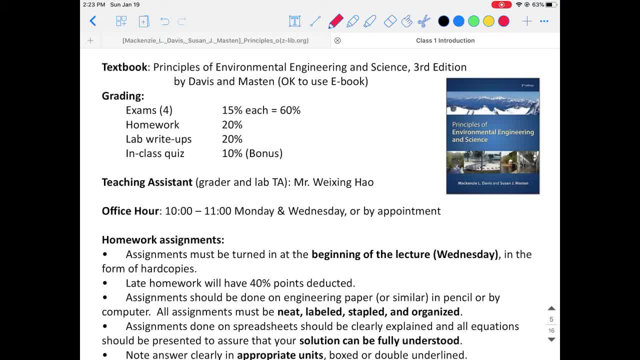 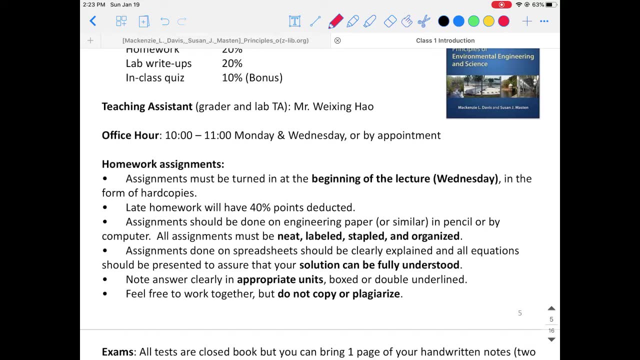 if you have other things going on during this period of time. okay, so you can either contact me. as I said, you can either contact me or contact Wei Xing. some requirements for the homework exams. so all of these exams must be turned in at the beginning of the lecture. so I'm going to give you the assignments on Wednesday. 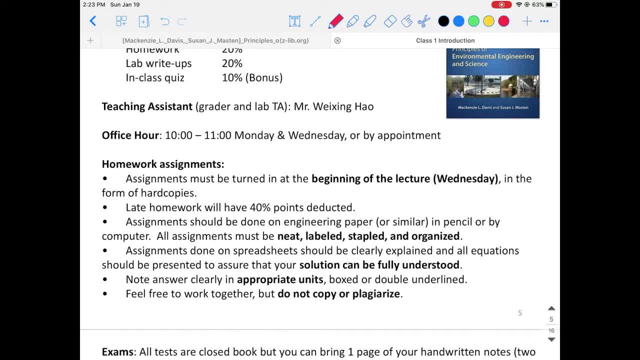 and for that reason it's due on Wednesday, basically next Wednesday, of the class, and it has to be in the form of hard copies. okay, and for all of the late homeworks, they will have a 40 percent of the points deducted. okay, and the assignments should be done on the. 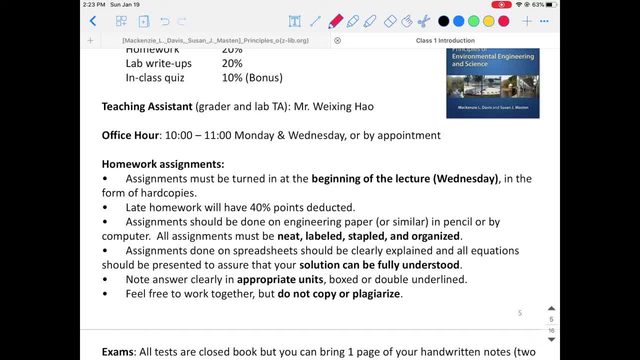 engineering paper and it should be neat, labeled, stapled and organized. and also for these assignments. I want you to not only calculate number, you have also have to give me the or demonstrate the solutions you have. okay, so it has to be understood, unless you think that the problem is too easy. but 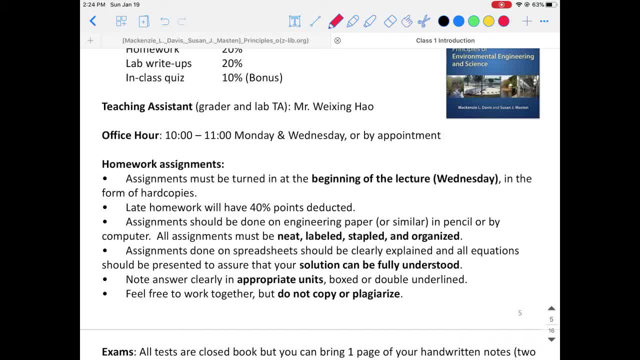 you can still come up, come to me and explain how you do that, okay, just by by talking to me. otherwise I don't think either me or the TA Wei Xing will be able to understand you if you just to write up a number there and also you need to know the answer clearly in the appropriate units. so during this class- because 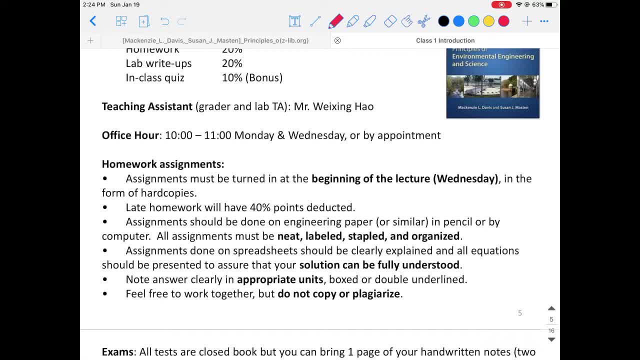 we're dealing with all different systems, so you're going to learn a lot of units there, and you? I want you to note all of these answers in the appropriate units. okay, and feel free to work, to work together, but do not copy to plagiarize. I don't think I had to mention this more in my class. okay. 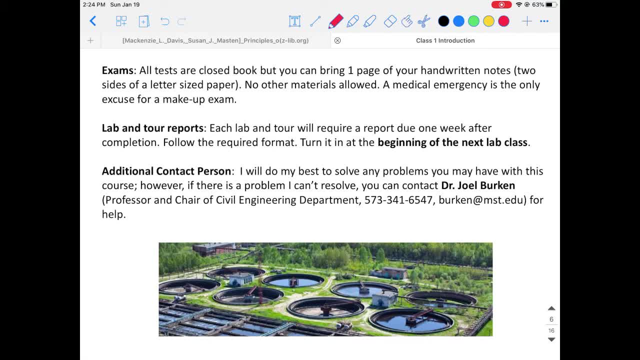 so, regarding the exams, all the tests are closed book, but you can bring one page of your hand region notes. it can be two-sided, because I think that it's going to be a little bit difficult for me to check your handwritten notes right before the exam, so you can write. 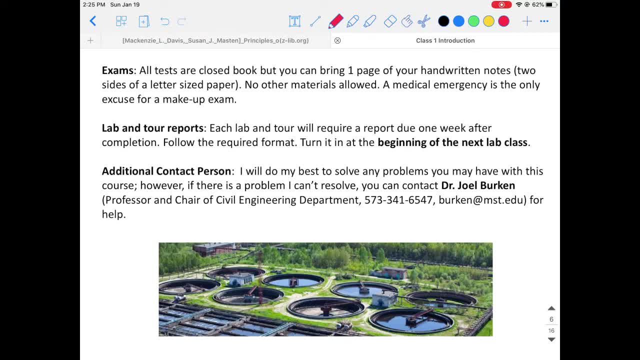 that one page. bring that with you to the exam. okay, no other materials allowed and maybe for one or two of the exams you can bring your calculator. that means that there are some calculations in in the exams, okay, and in terms of lab and tour reports, so you can see that, uh, the lab. 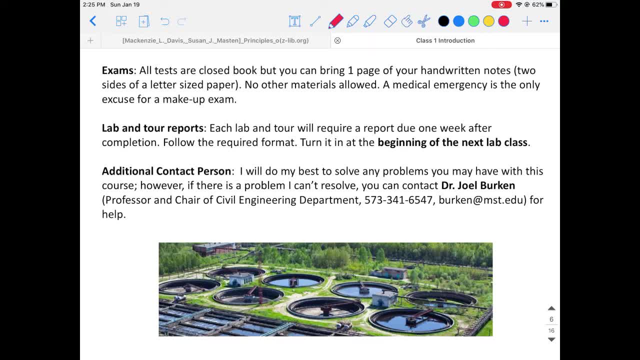 sections of the lab. okay, so you can either choose the Wednesday lab or the Thursday lab, and each lab and tour will require a report that's due one week after the completion. okay, so you should follow the required format and turn it in before the next lab class. okay, and for this class there are: 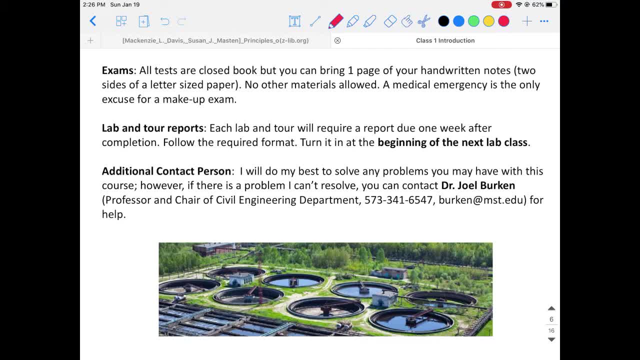 additional contact persons. okay, so I will do my best to solve your problems and I hope that you can enjoy this class. but if you are having a hard time following the class or you really hate me, you really don't like me, I say that this person, professor, is really terrible. or if you like me so much, maybe you like. 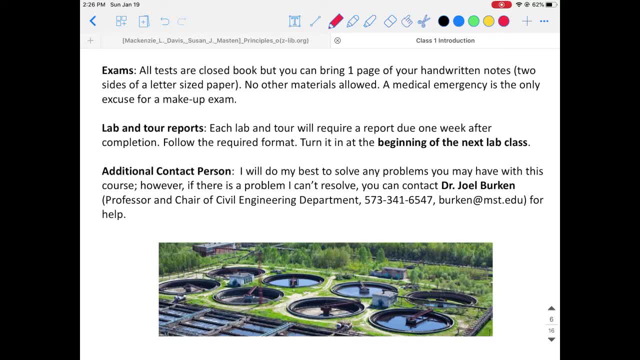 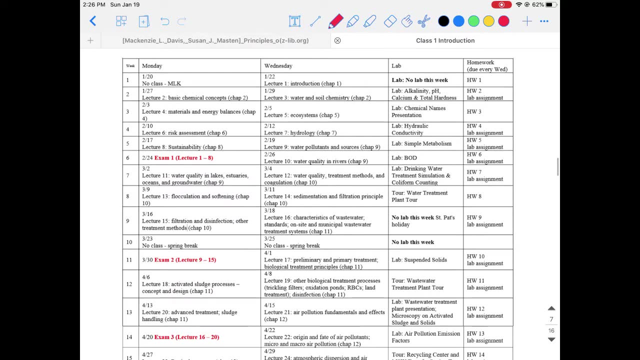 my teaching style or, like me, explaining things. you can also contact dr Joe Birkin, okay. so he's going to help you out. he's a chair of the department and he'll be able to help you with these questions, okay. so now, before we go, finally go into the contents. so here is. 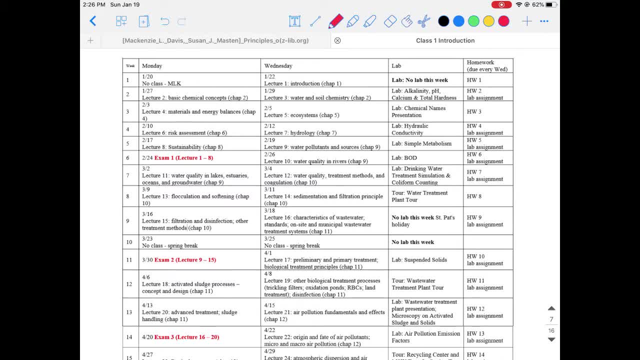 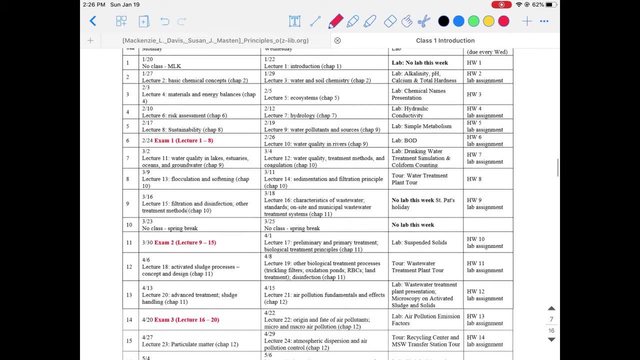 a rough schedule of our class. okay, for this semester the class is on Mondays and Wednesdays and then the labs are on Wednesdays and Thursdays, okay, so it also labels all the homeworks that's you that's due and all the lab assignments. 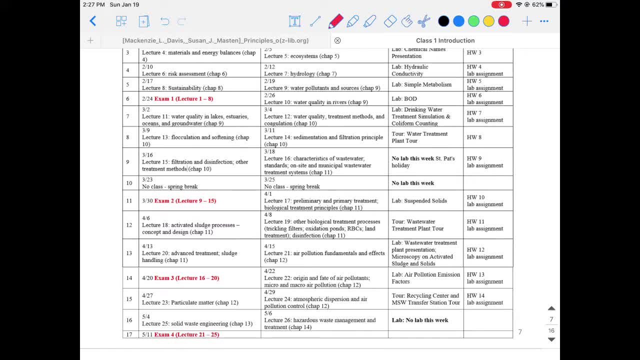 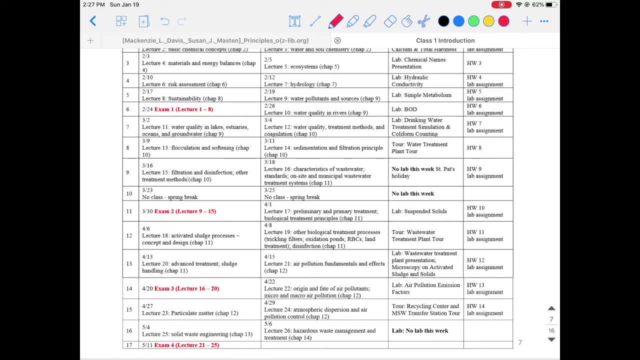 okay, so it also labels all the homeworks that's due and all the lab assignments. it also has the dates for the exams. so unless there are some extreme conditions, the exams are going to be taken on the dates labeled here. so you have to plan your time, schedule your time, really well. all right, and I also 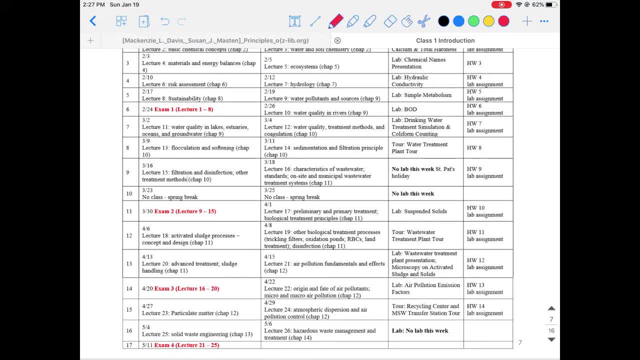 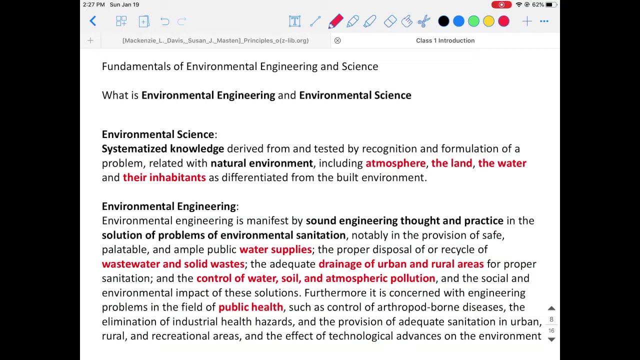 need to mention in advance that due to some other reasons, there might be that for some time that I'm not in town. so dr Dan Arthur will be able to help me cover some of the classes. so we'll find out, okay. so, as you have noticed, the name of our class is called fundamentals of environmental. 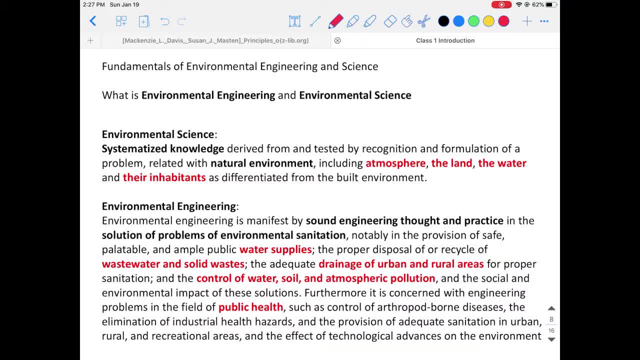 engineering and science. okay, so what is environmental engineering science? that's more specifically, what is environmental engineering and what is the environmental engineering, environment, environmental science? so whenever we talk about science, it's some knowledge, right, some theories there. so specifically for the environmental science, it is the systemized knowledge. 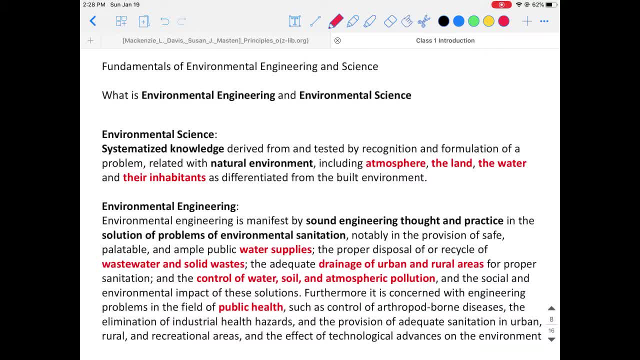 that are derived from all different sources but are related with the natural environment. it can include the atmosphere right, the land, which means the soil, and also the water and their inhabitants, as differentiated from the built environment. so there are natural environment and the built environment and we are interested in the natural environment and in terms of the 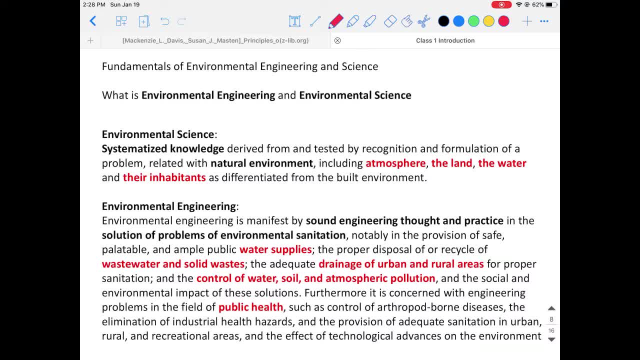 environmental engineering. so, basically, engineering is the applied form of the science. okay, so we're trying to build some devices to treat certain processes. okay, so the environmental engineering is the sound engineering thought and practice in the solution of the problems in environmental sanitation, and these problems can include water supplies, wastewater and solid waste, drainage of. 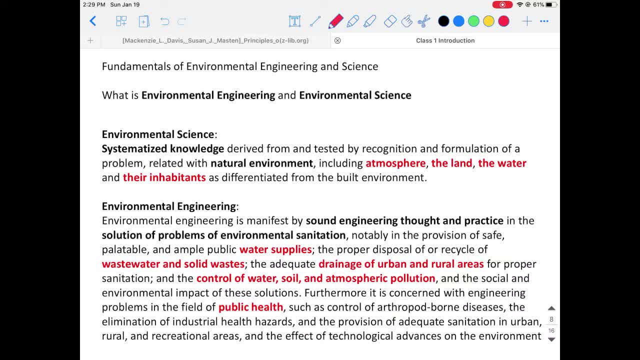 urban and rural areas, control water, soil and atmospheric pollutant and pollution and it also can relate with the public health. you can control the air, water pollution and it also can relate with the public health. you can control the air diseases and also problems related with sanitation. You can see that the environmental engineering is. 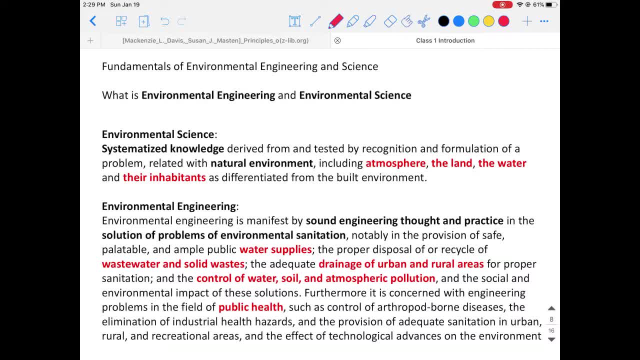 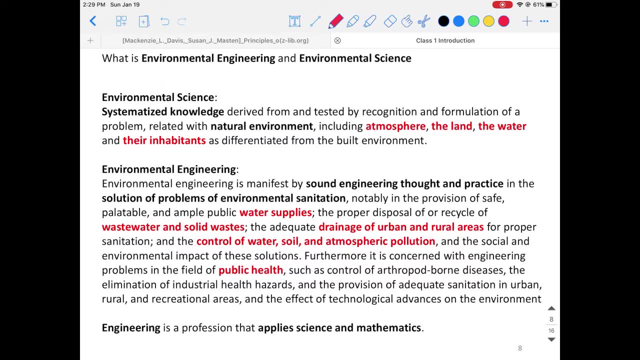 more targeted at the problems and we're trying to find engineering solutions by using these science or systemized knowledges here. So in short, you can see that engineering is a profession that applies science and mathematics. It applies for all the engineering and science subjects. 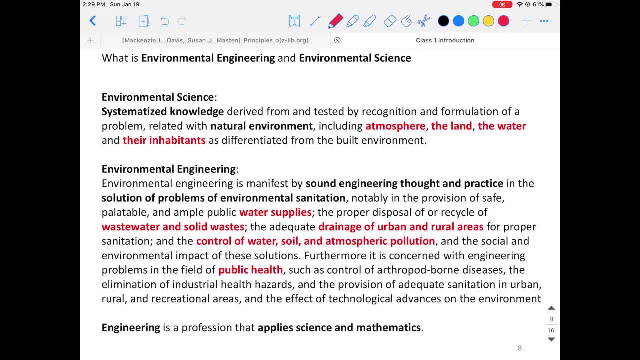 So then we may wonder what happens if we do engineering without science. No one likes doing these chemistry or physics. What about we do engineering without the science background? So here I have an example, and that's specific for the environmental engineering. Okay, 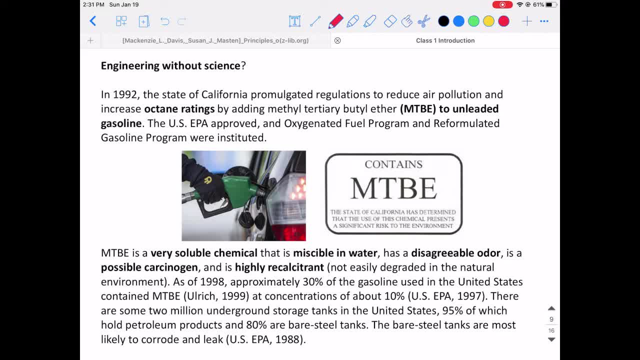